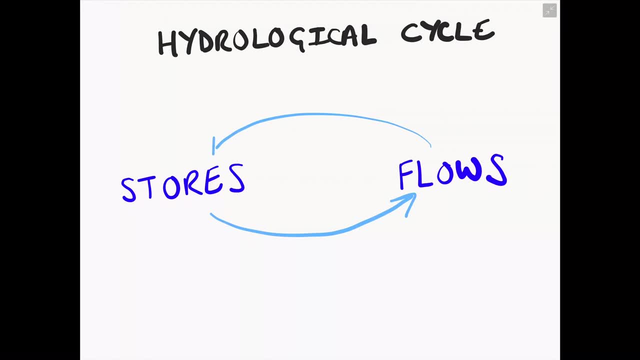 of water are where the particles, maybe a gas, a liquid or a solid- stay in that state for a period of time, So that could be, for example, in the ocean or the sea or a river. It stays as a liquid form for a certain period of time. That is a store of water, A flow of water. 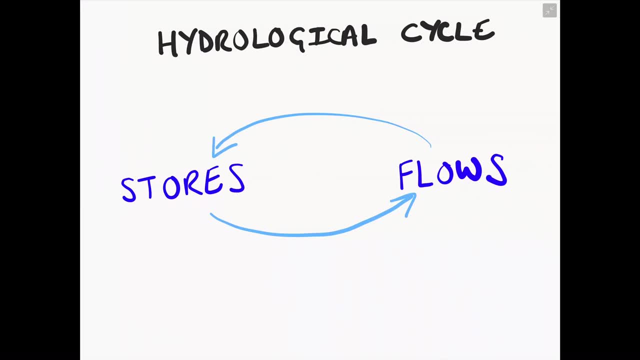 is when it moves from one state to another and it might change state or stay the same state. So, for example, when we heat water up from the sea, it will evaporate and it will condense and form a cloud. Now, in order for the water to move, whatever state is- in solid, liquid or gas- 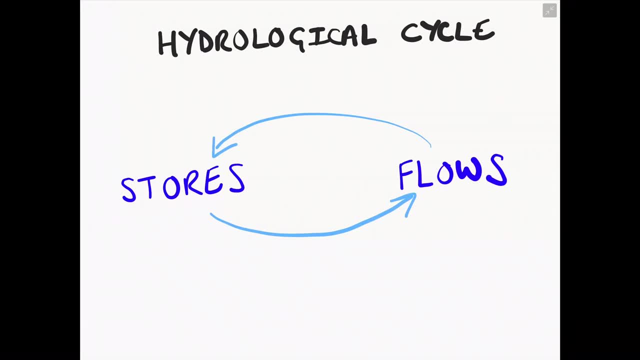 from your sea to your cloud, it needs to go through the two flows of evaporation and condensation. So let's take the time to go through the entire process of the hydrological cycle. Let's start off with a body of water. Now your body of water could be a sea. 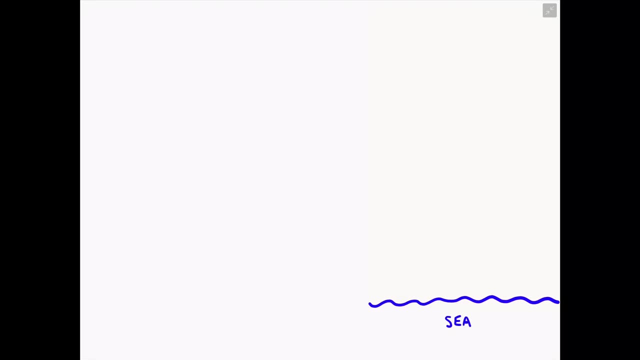 it could be an ocean, it could be a river, it could be a lake, it could be a puddle. It just needs to be a store of water that is kept in that same place and in that same state, in this case liquid, for a period of time, Over time, as this system is driven by the energy from the sun. 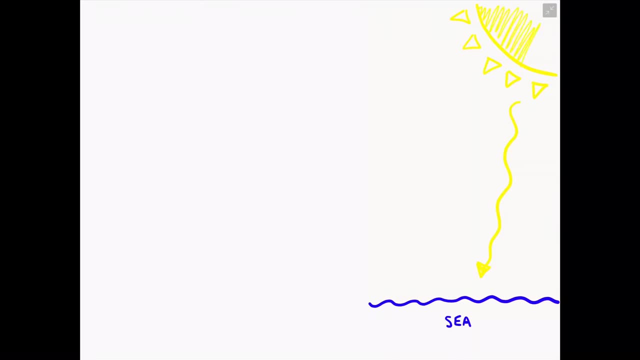 the sun will send solar radiation to that body of water and it will start to heat it up. What we then have is this store of water starting to transfer into a flow of water through the process of evaporation. So in this particular example, the sea- this body of water is being heated up so much that the 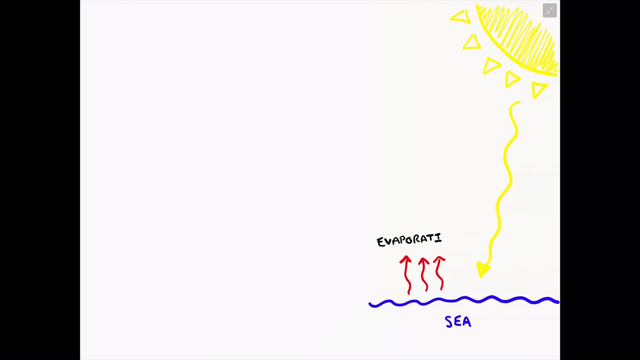 water particles are turning from a liquid into water vapour, which is known as a gas, through the process of evaporation. As this water vapour begins to rise into the atmosphere or the sky, it will cool down and it will start to evaporate. So in this particular example, 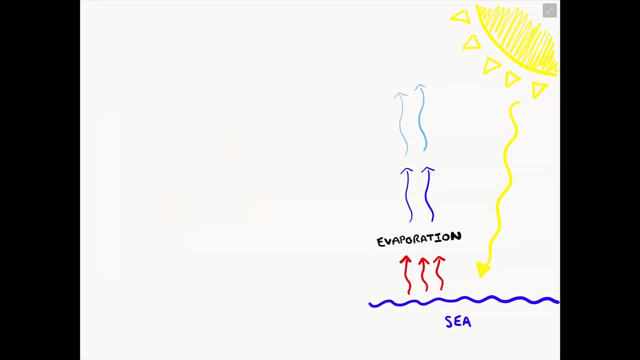 the water particles are starting to cool down and begin to form condensation. These water droplets are beginning to cool down because they are leaving the Earth's surface, where the solar radiation is the most concentrated and warm. That is why, when you go on aeroplanes, for example, 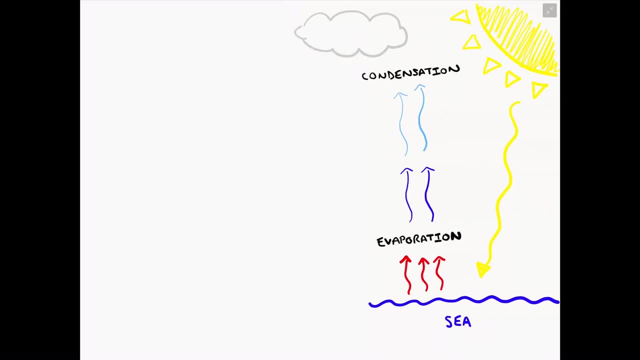 it is always a little bit colder because you are high in the atmosphere. The process of condensation then starts to join these water particles together, which then, as the water particles are cooling down, they are starting to form condensation. then eventually, when collecting enough, will form clouds. so clouds, in this case, is your next store. 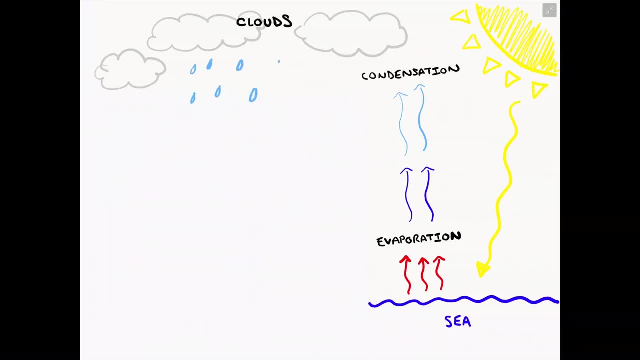 in the hydrological cycle. when these clouds get large enough and the water vapor becomes too much for the clouds to hold, the cloud will eventually give out precipitation, and precipitation can be in the form of rain, it can be hail, it could be sleet, it could even be snow. 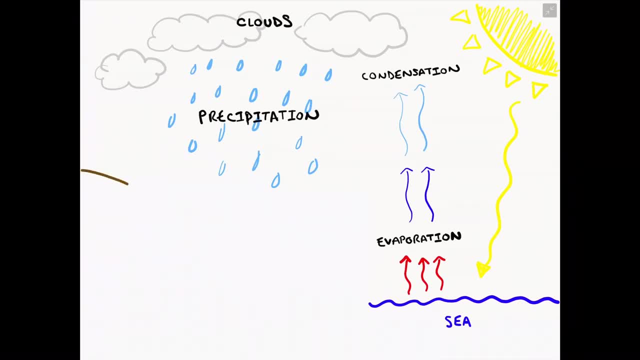 with precipitation being our next flow in the hydrological system. it will mean that, obviously, this water vapor in a liquid, or maybe even a solid state in this case, will begin to reach the earth's surface again, and it has three different options when it reaches our earth's surface. for one, it 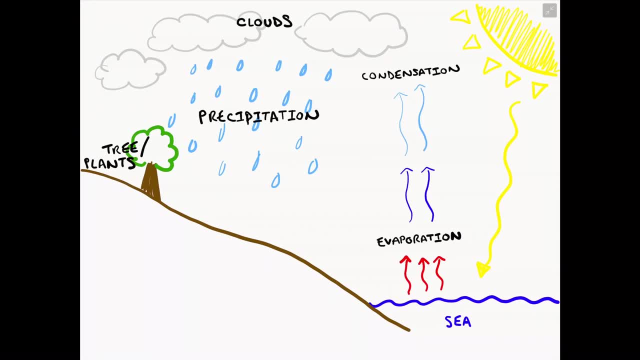 could come into contact with trees and plants, which would actually maybe hold and collect some of this water in the hydrological cycle, and then it would then be able to reach the earth's surface hydrological cycle. Alternatively, if you ever yourself have stood under a tree, when it is. 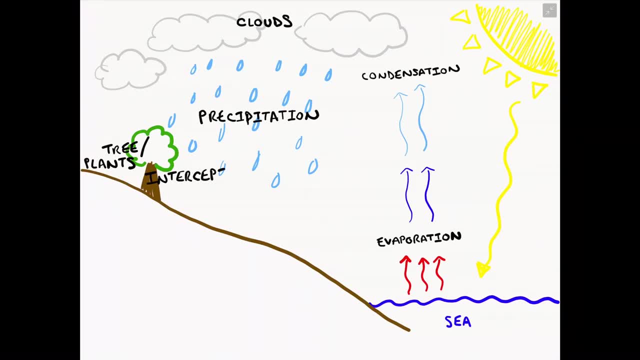 raining trees provide great interception, which is basically like a big umbrella that will stop the precipitation from hitting the ground, So it will collect maybe on the leaves of the trees, so it is intercepted When these water droplets or this liquid will actually hit the leaves. 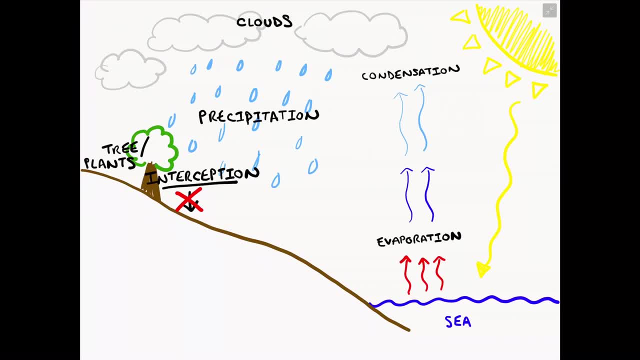 it might stay on the leaves of the plants or the trees for a period of time, So they are sometimes known as stores of water, And they might even themselves have evaporation from the leaves. the water might heat itself up from the energy from the sun, and it might go back into the 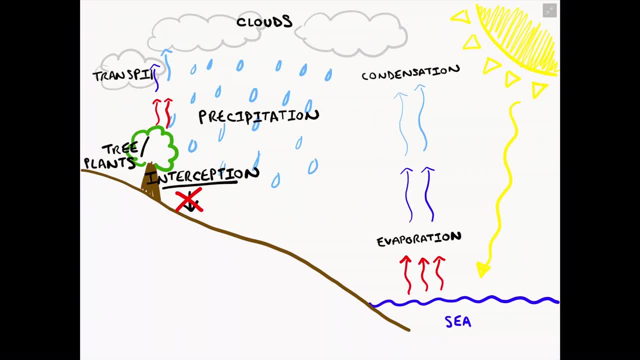 atmosphere, And we call that transpiration, this idea of evaporation from the leaves of the tree. Okay, so we've got another flow there. Now, if the precipitation does not come into contact with trees or plants, it might instead come into. 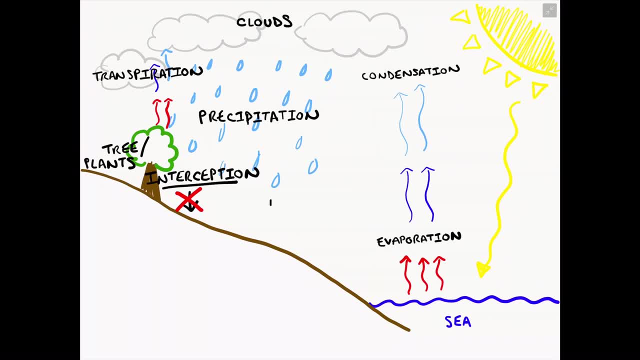 contact with the ground surface. So if we have precipitation falling to the ground, it might be that it comes into contact with tarmac or concrete or a road or a driveway. Unfortunately, these types of materials are known as impermeable: They will not let the water. 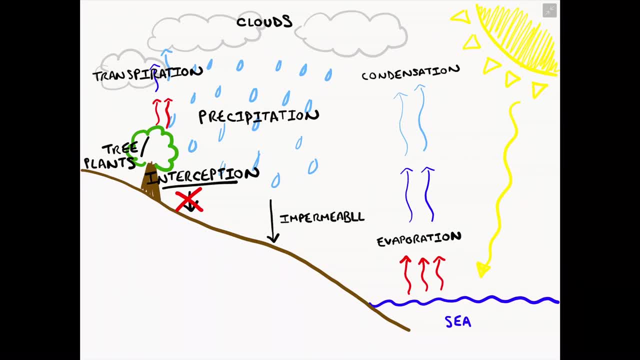 particles get into contact with the ground. So if we have precipitation falling to the ground, the water particles form or infiltrate or go into them. they are impermeable, which means that the water has no other choice but to run over the land surface, known as surface runoff, And this 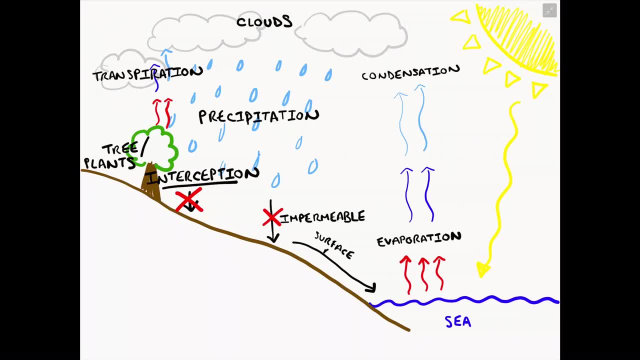 water might lead itself into drain pipes if it's in an urban area. If it is in a rural area, it might collect in a lake or go to a river, But eventually it's going to lead back to a body of water- a river, a sea, an ocean- through surface runoff. 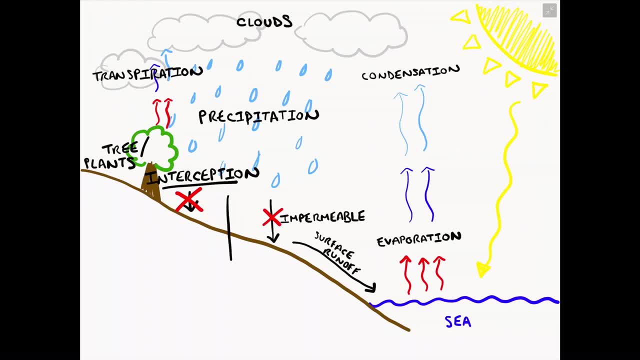 Alternatively, this precipitation could actually fall onto ground which is permeable, such as clay, sand grass. What this type of surface will do is allow the water to infiltrate, to soak into it like a sponge. So this permeable ground will actually absorb some of the water from the 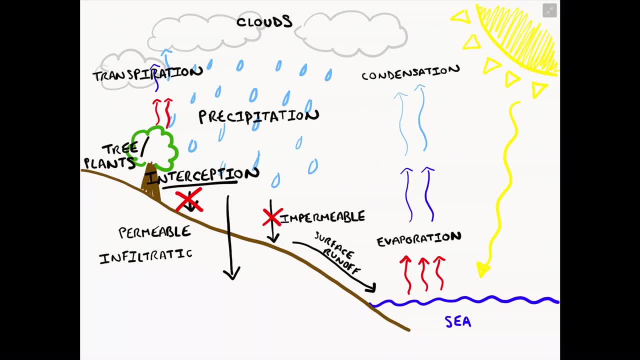 precipitation, and it will allow it to filter into the ground through the process of infiltration. This also means that soil and rock particles and sand are actually a store of water. If you yourself have ever walked on grass after it has rained, you might notice sometimes that the water 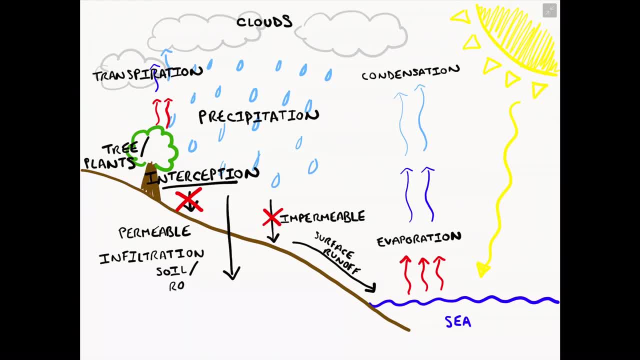 comes up through the soil back to the ground. So if you have walked on grass after it has rained, to the surface of the grass, and that is because the precipitation in the water, the liquid, is being held in the soil as a store. Now, once this water has infiltrated the ground, it might choose to do.